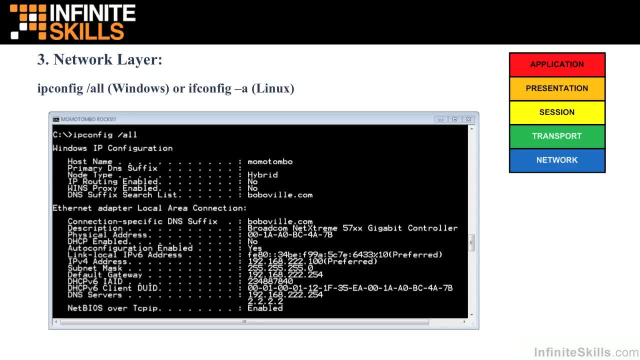 type in ipconfig forward, slash all, and we can identify the host name of the computer. In this case it's momotombo. The domain affiliation is bobovillecom. We then, looking down below, we see the ethernet adapter, local area connection. We see the nature of the network interface card. 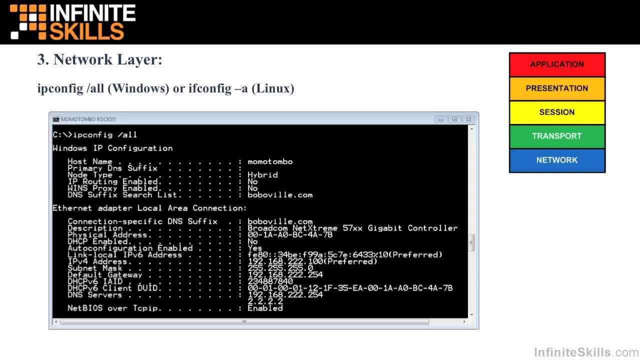 That's the manufacturer and the model number. Below that we see the something called the physical address. Now this is also referred to as the MAC address, The media access control address that is hard-coded onto this network interface card, So the first six characters of that MAC. 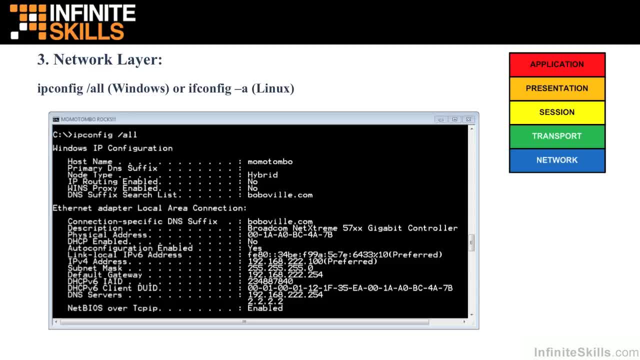 address represent the manufacturer and the last six characters of that MAC address are a unique value for this network interface card from that manufacturer, Defined by the first six characters. You notice these are 12 characters. in hexadecimal It's a 48 binary bit string. We scroll down a little bit and we see the link: local IP version 6 address. 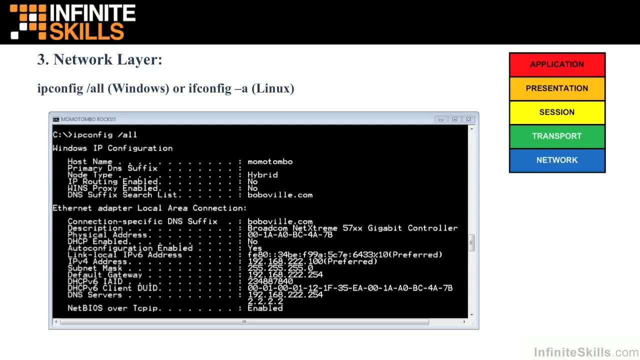 That's just for future reference. We're going to look at IPv6 in another lesson. We'll move down past that. Then we see the IP version 4 address, and in this case it's 192.168.222.100 and its. 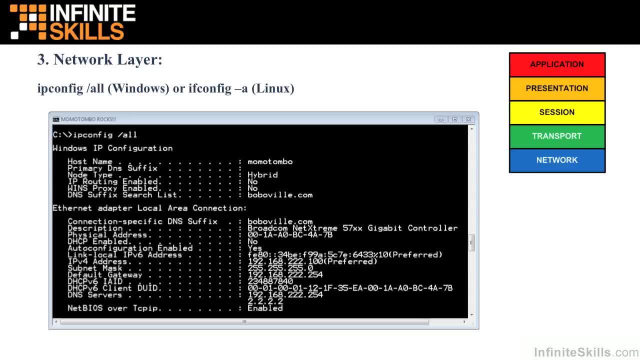 subnet mask is 255.255.255.0. that equates to a slash 24 mask. In addition, we see the default gateway of 192.168.222.254. and finally, down below, like the last two or three lines, we see the DNS servers and in this 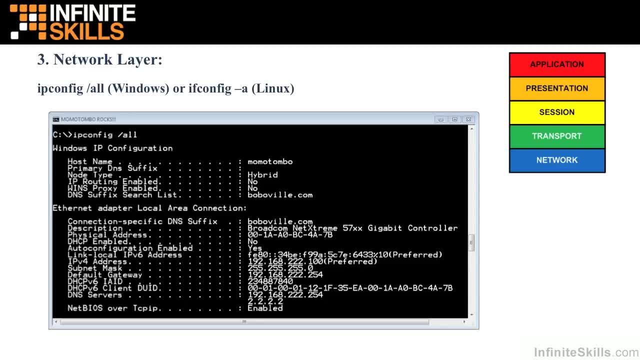 case to our listed 192.168.222.254 and also a second one at 2.22.2.2,. that's as if you're first dns server for name resolution at 222.254.. If that server is unavailable for any reasons, then go talk to the other DNS server at 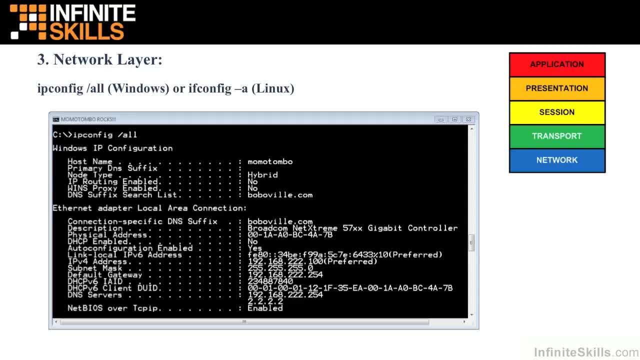 this 2.2.2.2.. Now that IP address is out on the public internet First, 192.168.222.2.54 comes out of the private IP address space. That would be a DNS server on the corporate network. The second: 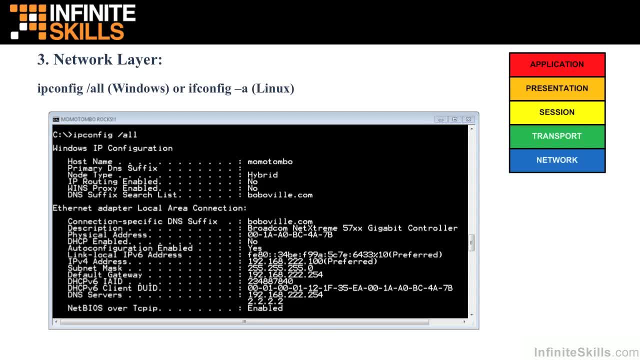 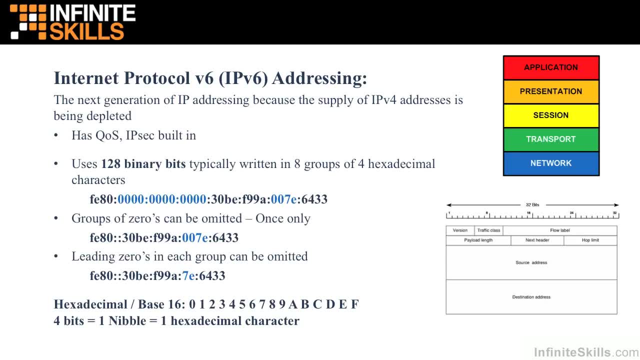 one is a DNS server out on the public internet. Moving forward, we're going to take a look at IP version 6, another layer 3 network layer protocol. Now, because we started running out of IP version 4 addresses, they have started generating and implementing IP version 6 addressing IPv6 uses. 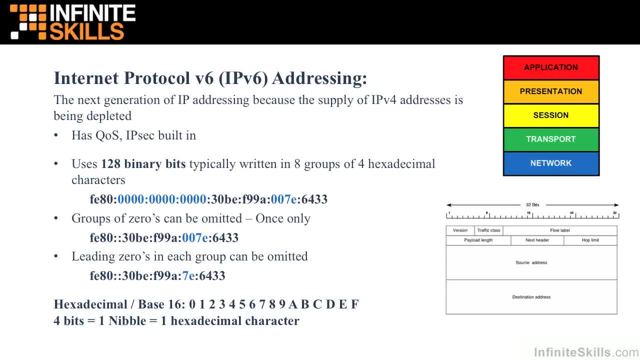 128 binary bits, in contrast to the 32 binary bits in IPv6. used by IP version 4.. So IPv6 is a much longer IP address and therefore we have many, many, many more addresses available that will allow us to continue to add servers and other systems onto. 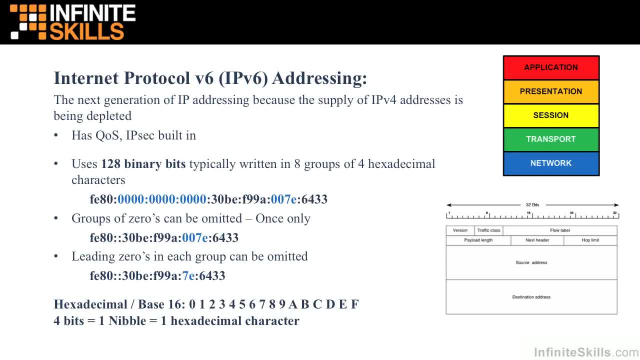 the public internet, Now IP version 6, because it's the newer version and it has a great deal more configuration ability because of its greater length. we can add extra services into IPv6. And one of them is called quality of service, which allows us to prioritize packets Typically. 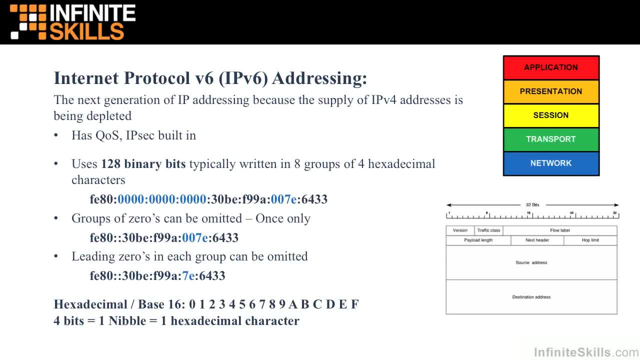 these would be time sensitive packets like voice and video. We can say, because this is time sensitive, let him go to the front of the line and let him zip through the network faster than other lower priority packets. So quality of service is generally for time sensitive packets. 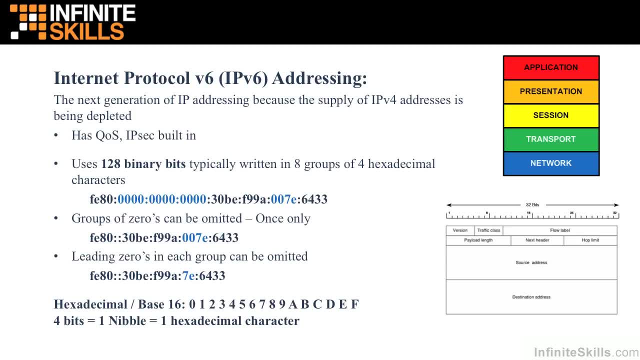 on a network and the infrastructure has to have the ability to recognize QoS. But then, if it does, knows how to prioritize these and let them go at the head of the line first. IPv6 also has encryption built into it. That was a weakness that IP version 4 did not. We had to generate a brand. 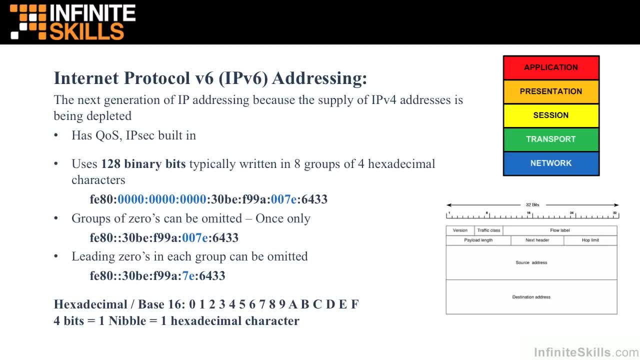 new protocol called IPsec, internet protocol security. that is different from IP in that added encryption to the IP packets. Now back to IP version 6.. IPv6 address, as you can see here in this example, is a IPv6 address. So IPv6 is a IPv6 address. So IPv6 is a IPv6 address. So IPv6 is a. 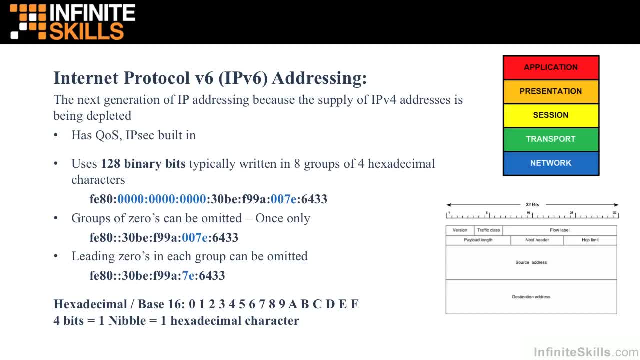 ISP, but it will call the IP system like an IPv6 address. We want to take a look at that because it's going to be a pretty big problem. So here's a few examples of IPv6 that we can use. This first example starts with FE80.. And then there's a whole series of zeros and et cetera. 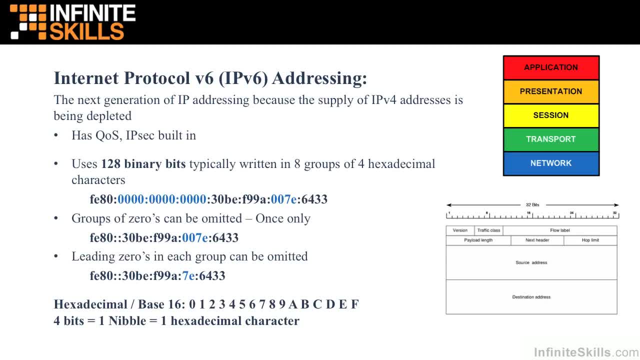 et cetera. So what we see is using something called hexadecimal characters. Hexadecimal is a numbering system that has 16 different characters, So I can count from zero to 16 without reusing any of the characters. What we see is that each section in an IPv6 address. 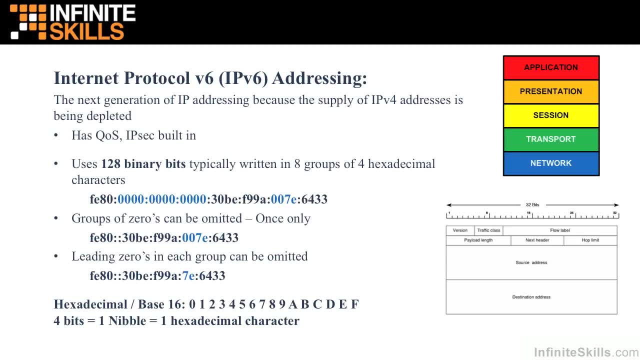 has four of these hexadecimal characters, and each character represents four binary bits, So I get 16 binary bits per section. That's a very long IP address and I'd hate to have to type that in more than once. However, what we can do with IPv6 is we can omit this long chunk of. 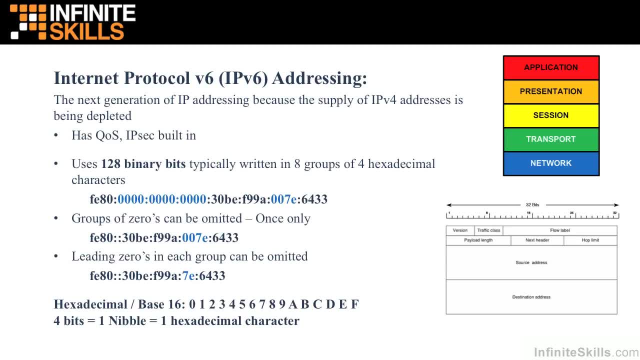 consecutive zeros And we simply omit these zeros and what we notice is a pair of colons side by side. So in this case we've left out those 12 zeros, but because we know that this address has to be a fixed length, we look for the double colon and we simply insert an appropriate amount. 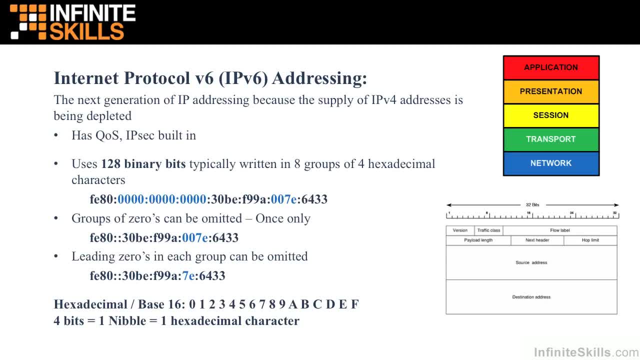 of zeros to make this the proper length. So we can omit the zeros to simplify the writing of an IPv6 address. Further, in each of these sections, we can omit the leading zeros. So, as we see this, one section has 007E. Well, if we look down towards the bottom, we see that we can. 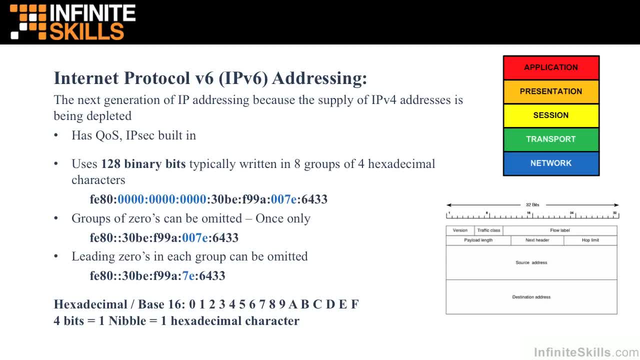 actually even throw away those leading zeros and that section simply has the 7E. Now the end user and of course the routing system and the nodes all must understand and actually automatically accommodate this by filling in any missing characters with zeros. So again we can do. 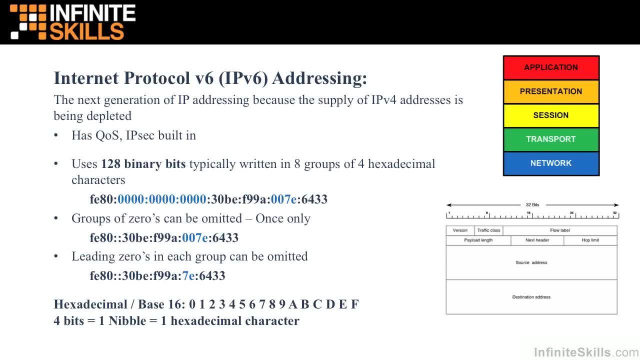 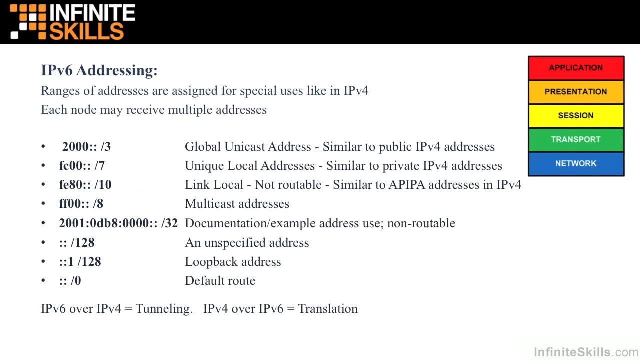 these two things to shorten the length of the written IPv6 address. However, the processing automatically adds all those binary zeros back in appropriately. So this is your IPv6 IP addressing. Now these addresses are broken up into different ranges, similar to the way IPv4 is broken up into certain ranges, and we have a public IP addressing called Global. 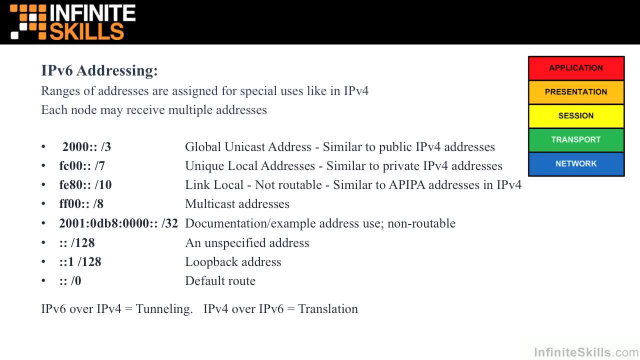 Unicast Addresses that started with a prefix of 2000.. We have Unique Local Addresses. This is equivalent to IPv4.0.. We have Unique Local Addresses. This is equivalent to IPv4.0.. We have Private Addressing and they start with FC00.. We have something akin to the Automatic Private IP.